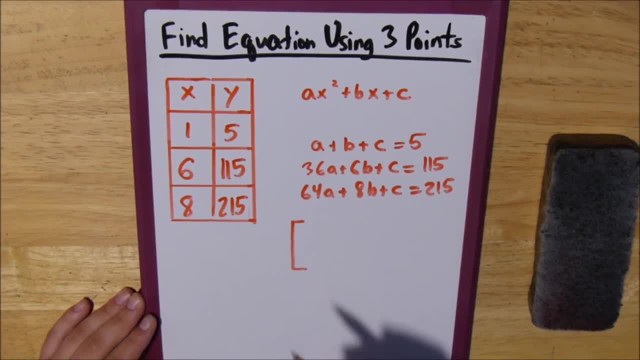 So our first value is going to be one. You basically just take the coefficient in front of a, b and c and you just put them there respectively, right? So we have one, one and one, Then we have 36.. 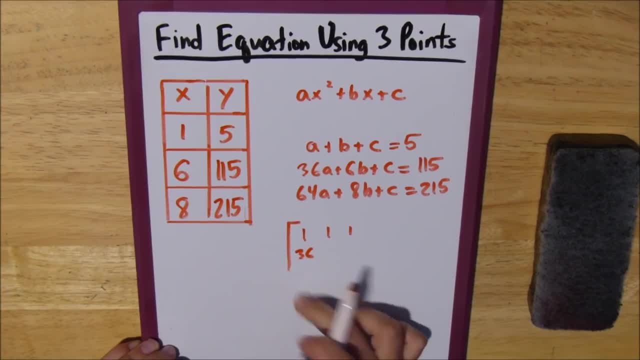 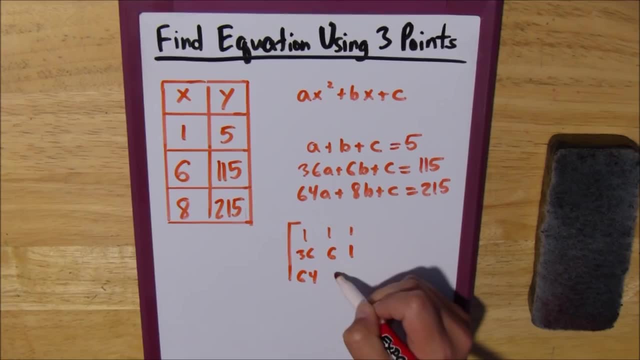 36,. I need to make this matrix bigger. All right, we have 36,, we have six and we have one. Then we have 64,. eight and one. Now notice that your c value is normally going to be one, okay. 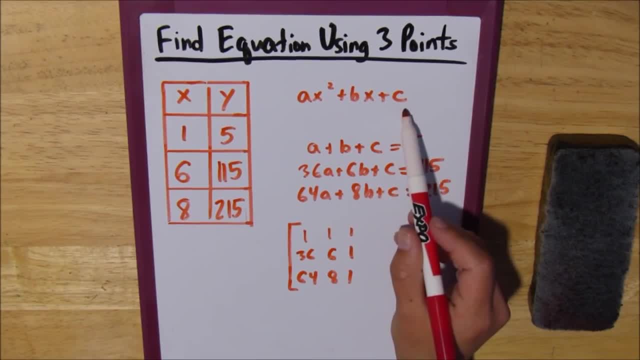 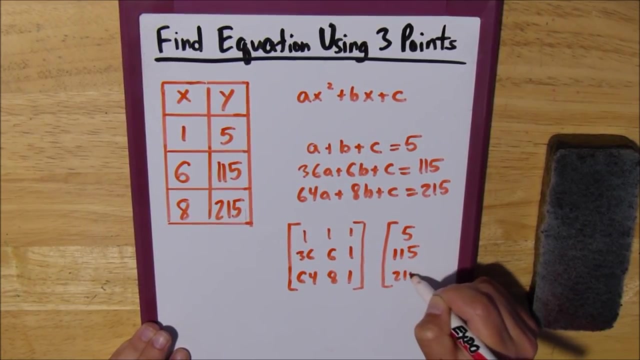 Because x is not. You're not multiplying c by x, right? So it's just going to be one, All right. and then our second matrix is going to be these y values Five, 115, and 215.. All right, now we're going to do what we call an inverse matrix. 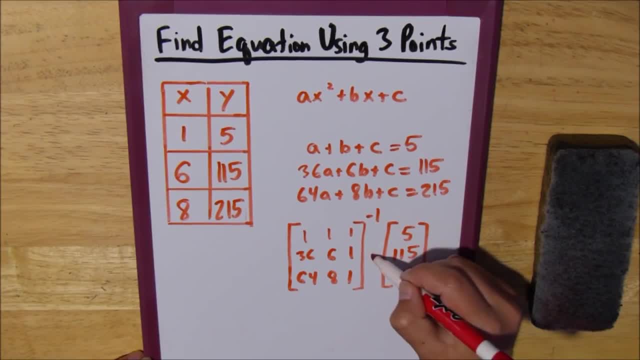 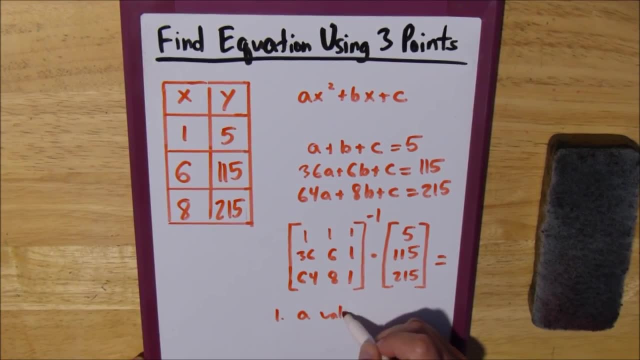 So you basically just raise this to the negative first and you multiply these together And what you should end up getting is the first number should be the a value, The second number should be the b value And the third number should be the c value. 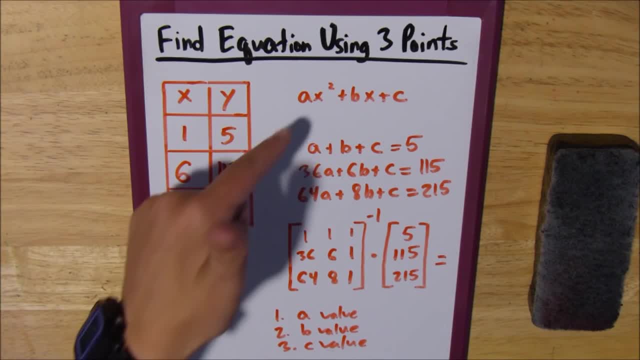 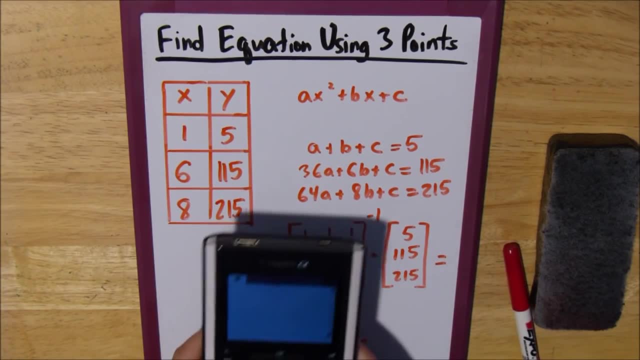 So if you know all three of these numbers you can figure out what the equation is right. So let me just get my calculator. So go to matrix C, three by three, Put in the first one, one, one, one. 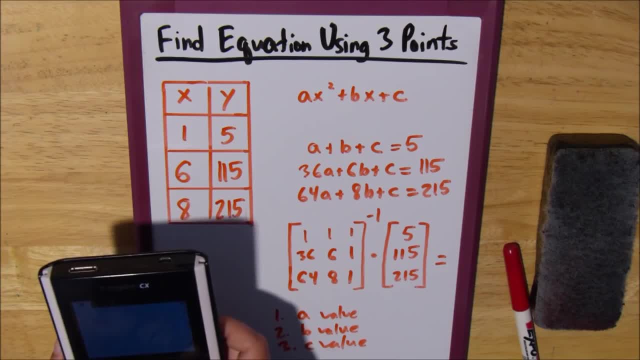 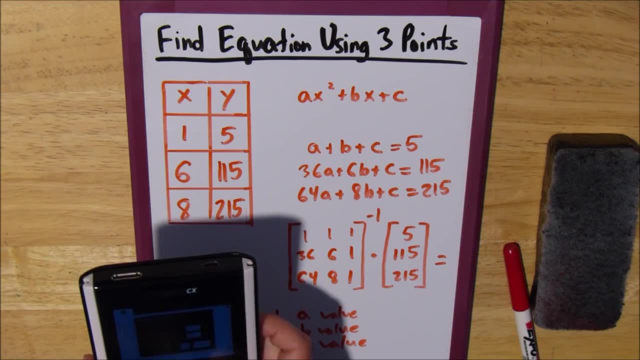 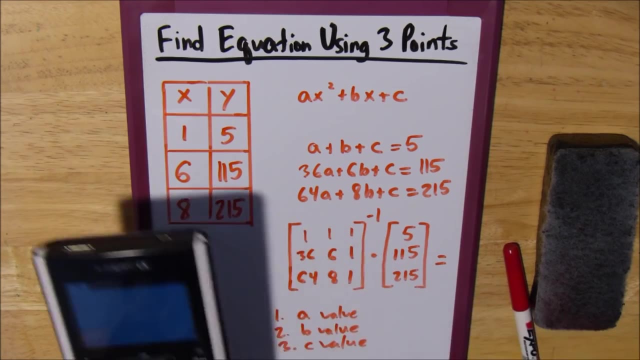 36, six, one, 64, eight, one To the negative first times number of columns is one. To anyone who's looking for a calculator, I'd really recommend the TI Inspire. TI Inspire CX. it's, it's in color, it's, it's awesome. 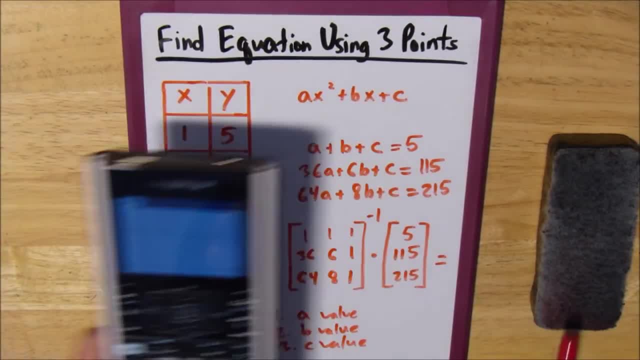 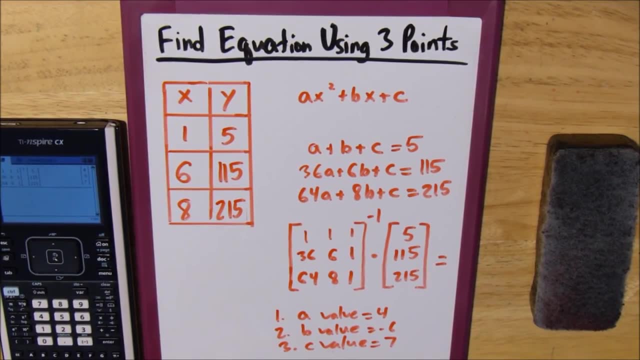 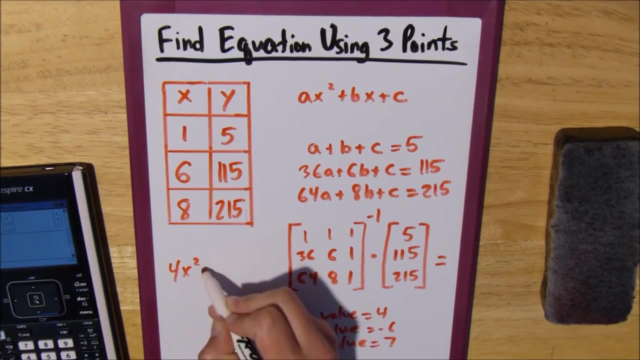 215.. All right, so I ended up getting a is four, b is negative six and c is seven. Now the fun part is we can, so let me just write out the entire equation. So four x squared plus, I suppose, negative six. whoopsie daisies. 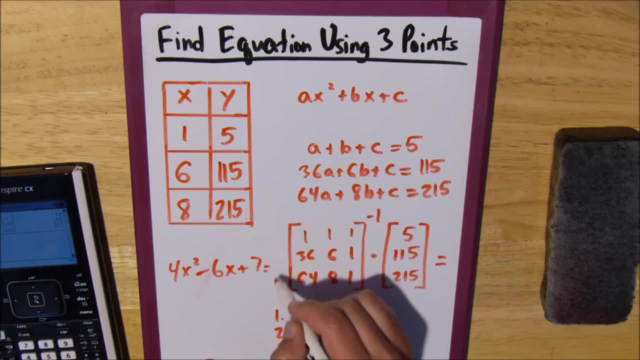 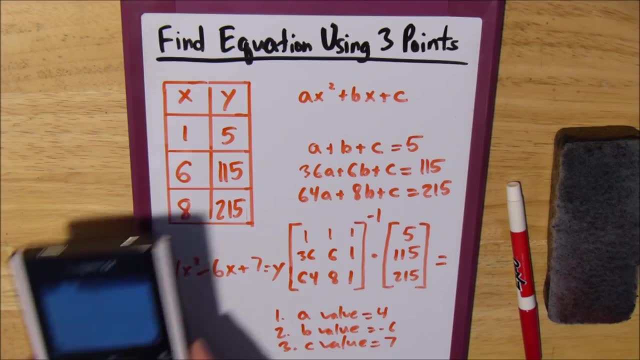 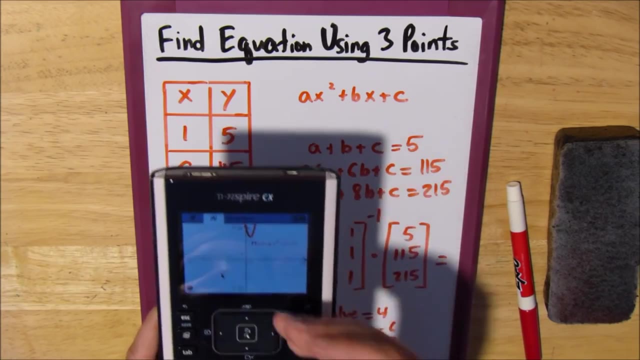 Negative. six x plus seven equals y. So now let's graph that. Oops, minus six x plus seven. All right, so the graph has moved up seven units. so let's just or not moved up seven units. moved up some units, but it's not seven. 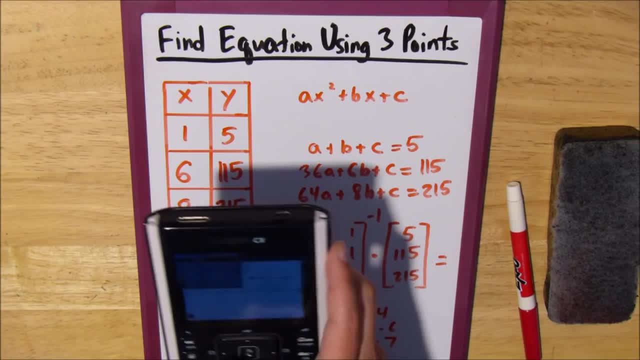 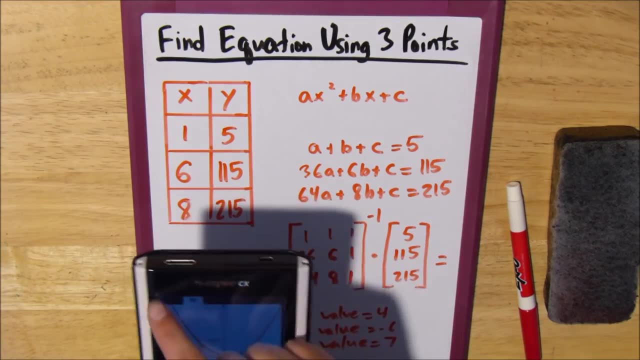 All right, let's go to view- and oh, that's not it window zoom and fit, So now you can see the the graph. but the really cool thing about this calculator is that you can see the table. So let's see our first x point was one. 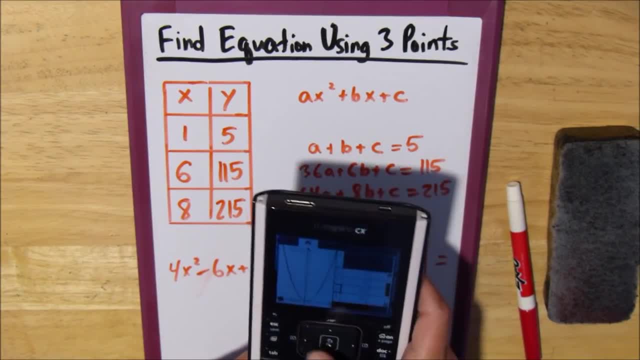 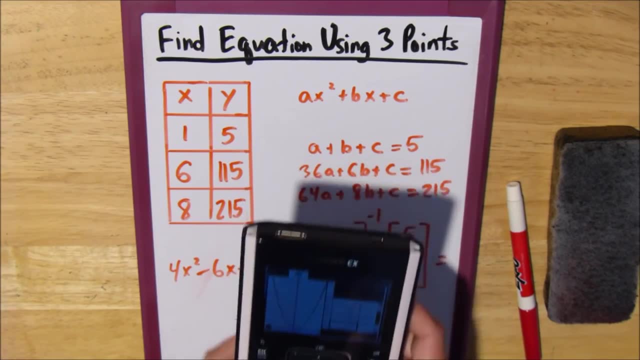 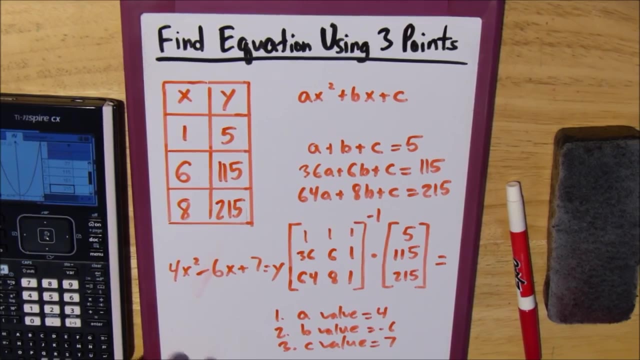 and look, it corresponds to our y point of five, then our second one is six, six and 115, then we have eight and 215,. great, So that means we have figured out the equation using matrices. Now, what if I told you we could just skip this entire part? 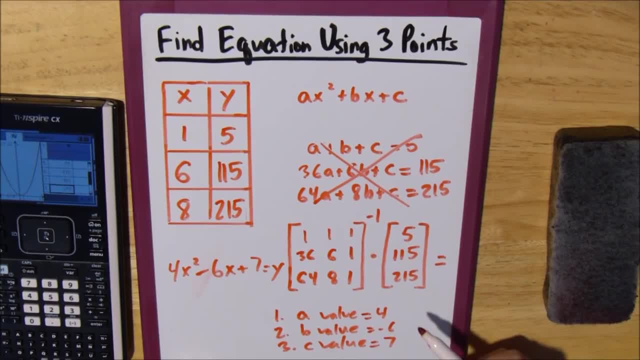 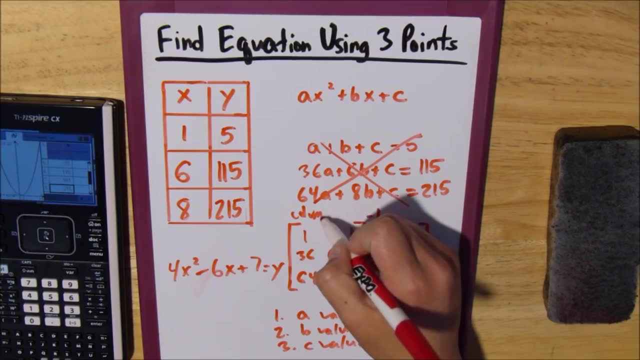 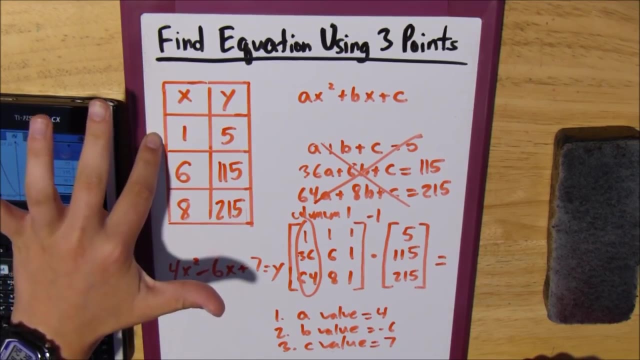 We wouldn't have to write out these equations, We could just skip right to the matrices. Well, you actually can. So the first column, column one, wow, okay, column one, this column here, you basically just take your x value and you square it. 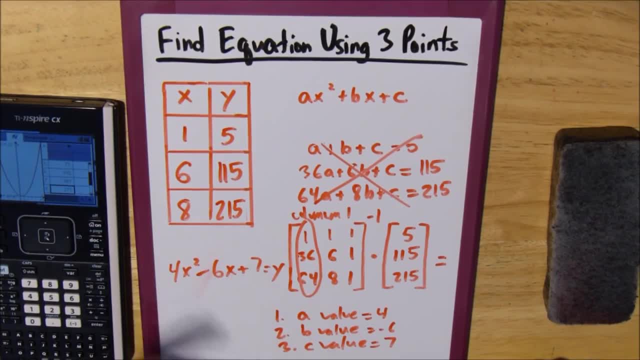 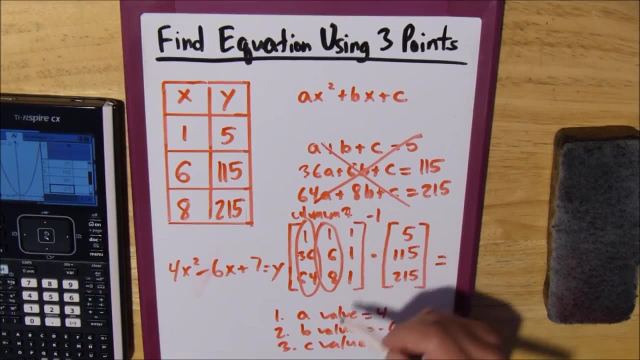 So one squared is one, six squared is 36,, eight squared is 64.. Column two: this one is basically just your x. So one, six, eight, And then column three is really just one. Your c value will never change. 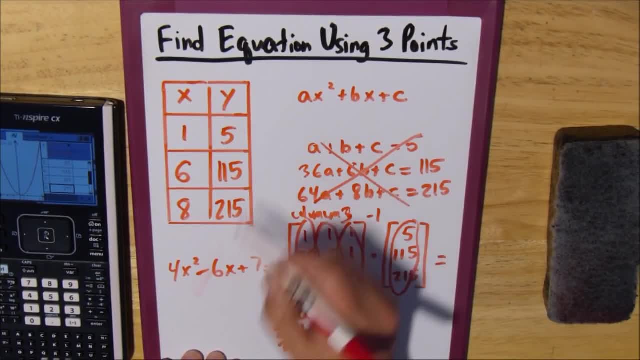 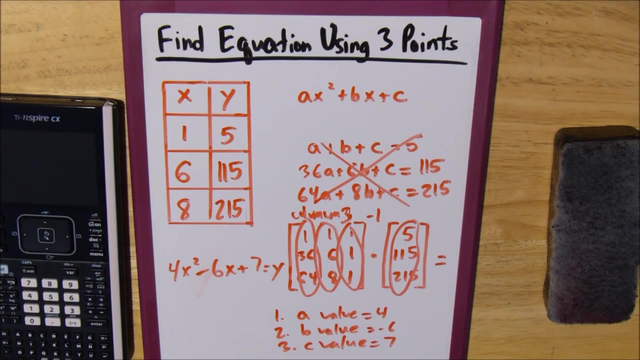 It will always be one, And then your second matrices would just be your y values, And that's basically. that's basically how you do it. It's it's really useful because, like I said before, quadratics aren't like linear and you can't. 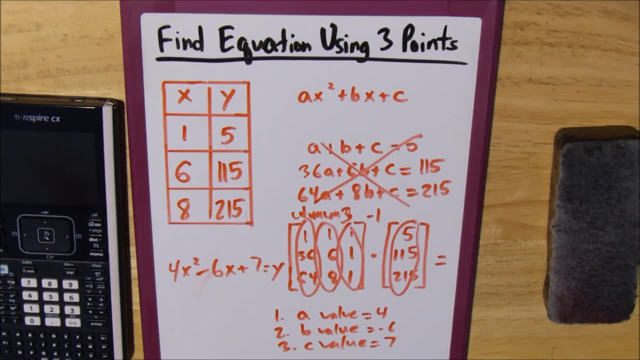 did I say that before? I'm not sure, but let me make the point that quadratics aren't linear, right, They're not in a straight line. They they have like a U shape. But matrices are a really cool way to figure out the quadratic equation. 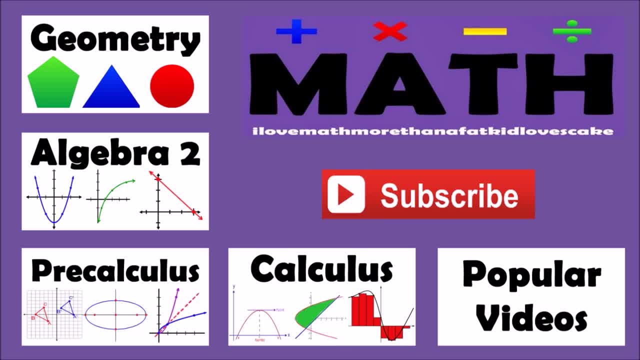 Ooh, it's the end screen. Click on one of these links to be directed to that playlist, And don't forget to subscribe.